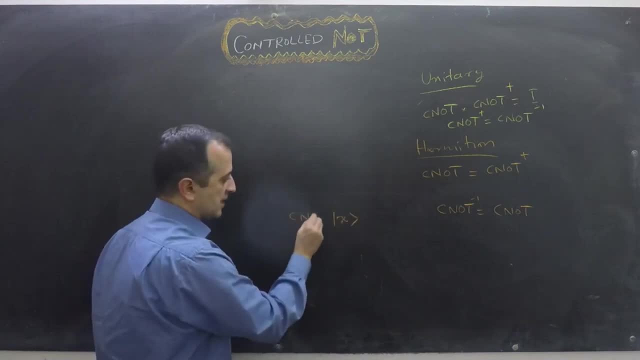 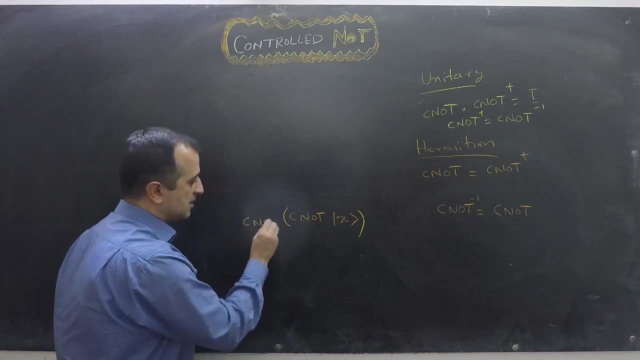 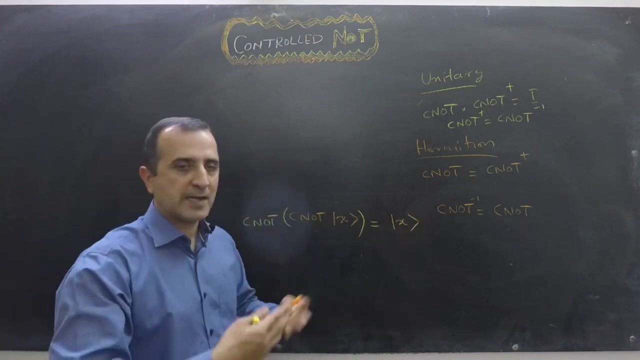 it is a two qubit gate and I apply CNOT on that gate And then, whatever the result I have, I apply CNOTE once again on the result. then my answer will be getX, which was the original input. That means input will remain unchanged because these two CNOTE will cancel. 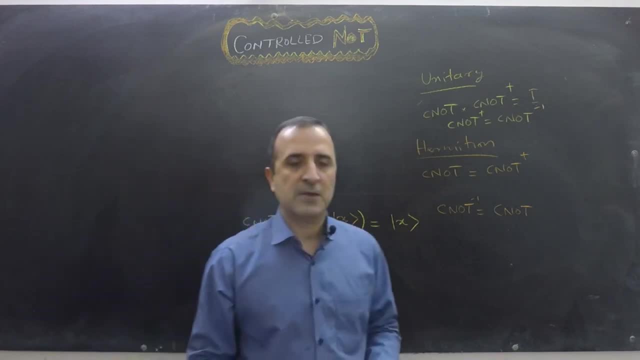 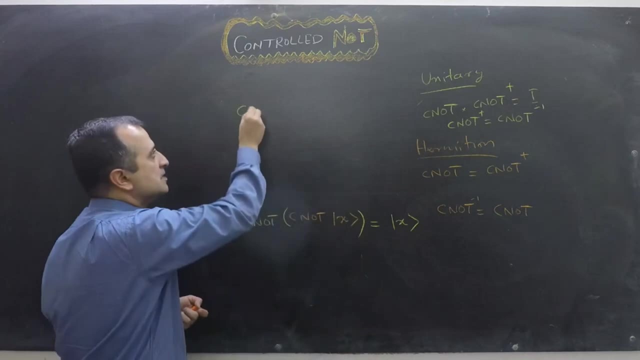 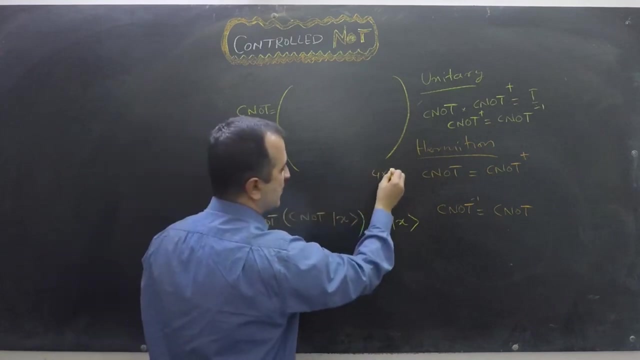 each other effect. Like all quantum gates can be expressed in a matrix form, so we can express CNOTE gate also in a matrix form. So in a matrix form, CNOTE gate in a unitary matrix form is expressed by a 4x4 matrix. And why 4x4 matrix? Let's say you have a single. 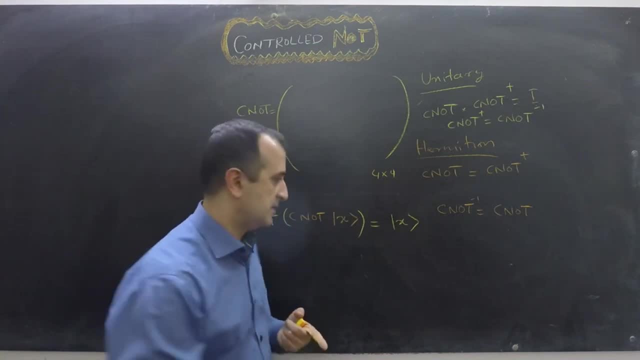 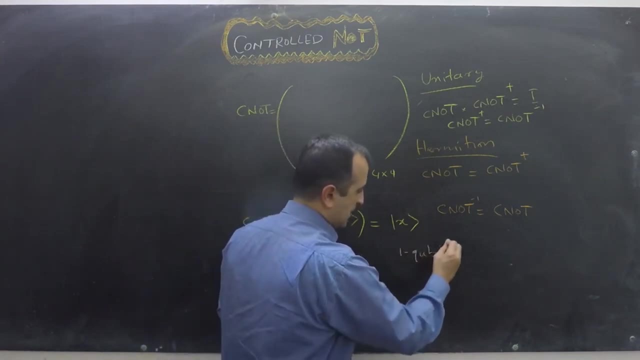 qubit gate. For single qubit gate you need 2x2 matrix because 2 raised to the power 1 is 2.. So for single qubit, for one qubit, we will need 2 raised to the power 1 times. 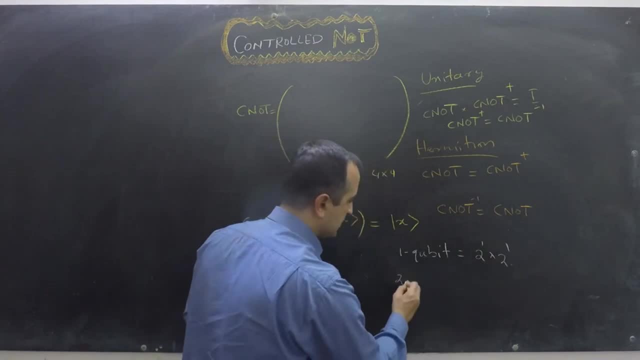 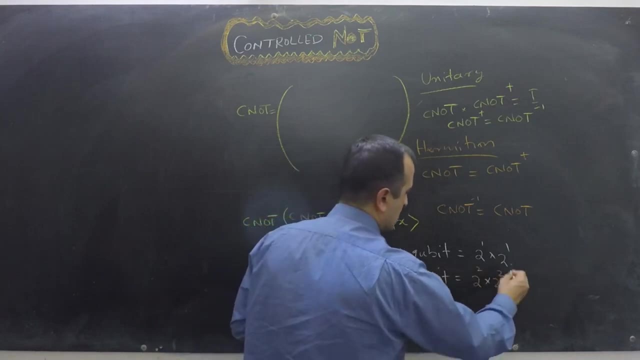 2 raised to the power 1. matrix For two qubits we need a gate which is 2 raised to the power 2 times 2 raised to the power 2.. And similarly, for n qubits we need a matrix which is 2. 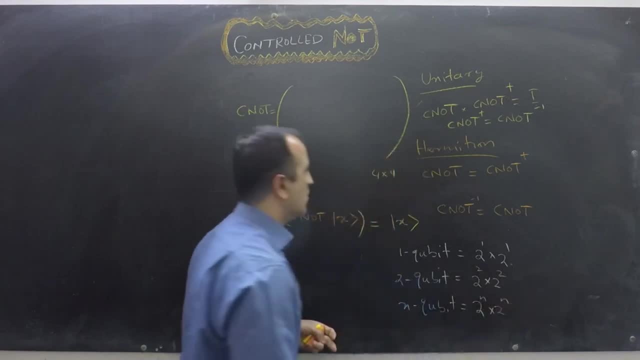 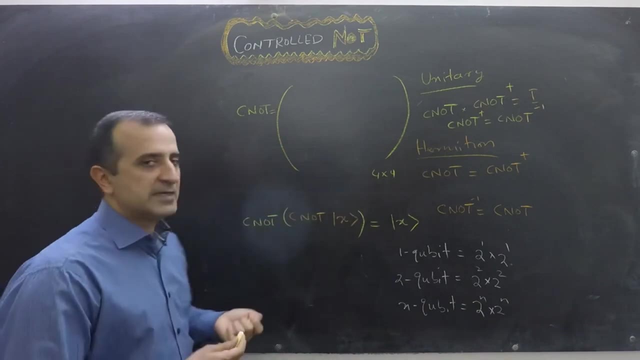 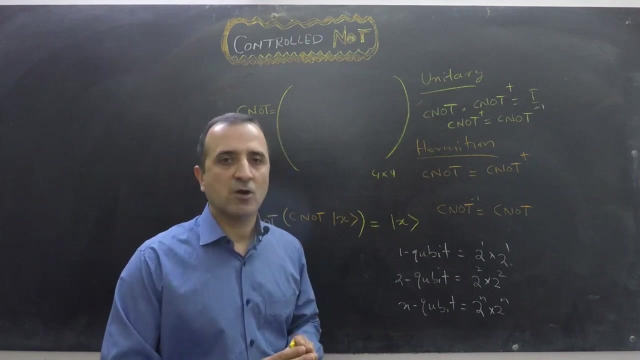 raised to the power n times 2 raised to the power n. So because it is a gate for two qubits, so it represents it as a 4x4 matrix. And this matrix is very similar to identity matrix. First two columns are the same as of identity matrix, but the last two columns are swapped. 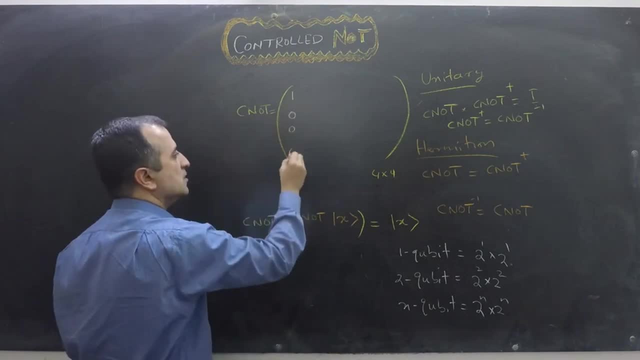 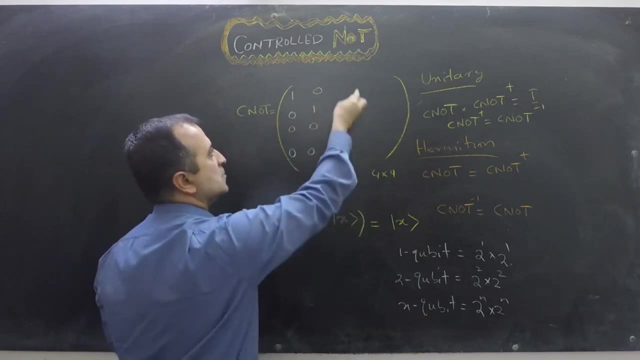 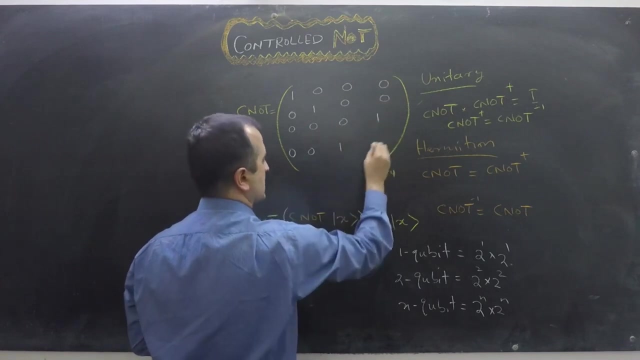 So the first column is 1 0 0 0. 0. second column is 0 1 0 0, and these two last columns are swept with each other. so we will have here 0 0 0 1 and we have here 0 0 1 0. so now why it is called. 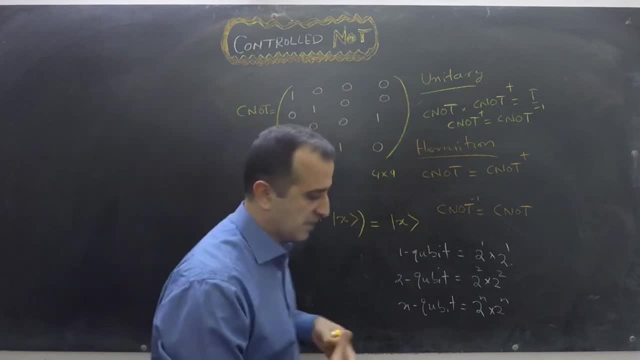 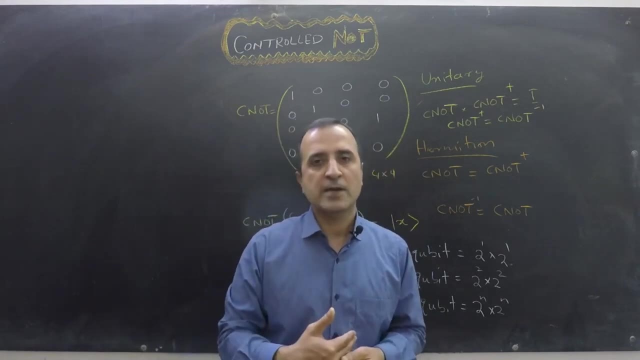 control node gate. it is because, in general form, in simple form, the first qubit represented as a control bit and if the first qubit is 1, then it flips the second qubit. if the first qubit is 0, then the second qubit remains the same. 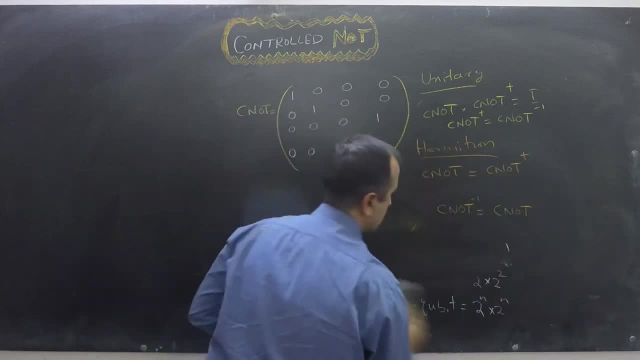 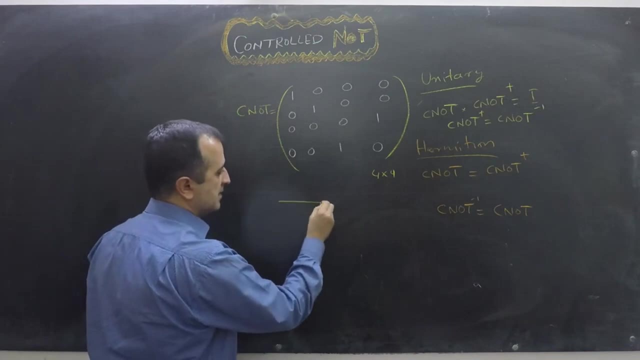 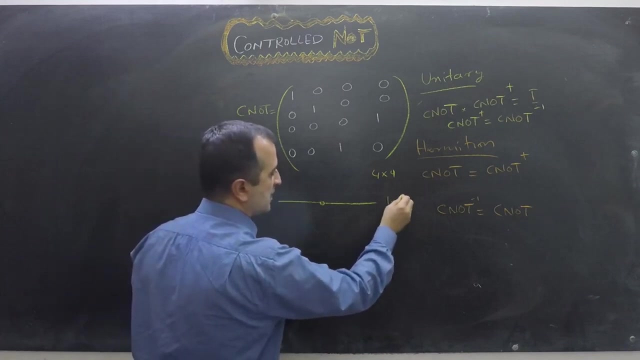 let's see what that means. so in the general form we can say that this is a representation of CNOT gate. then the first qubit- let's say it was X or input, it will be on the output, it will also be the cat X. and the second qubit depends upon the first qubit and that means the second. 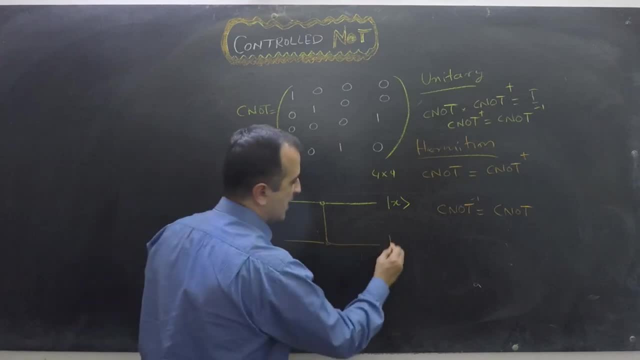 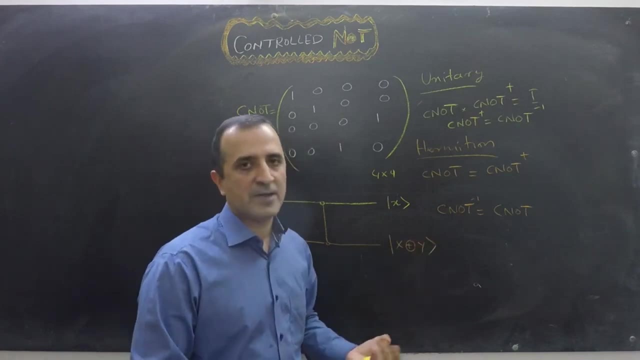 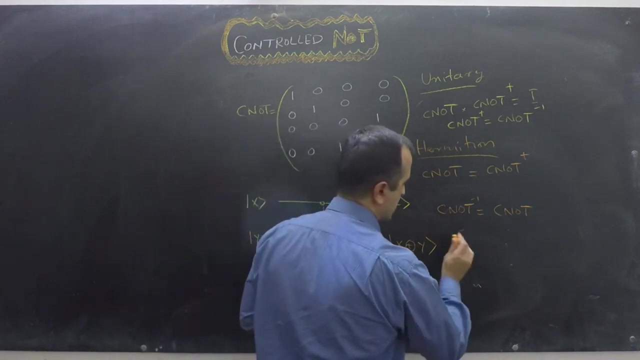 qubit is Y, then on the output and we will have X exclusive OR with Y. and we know: when we do XOR with 0, our result remains the same. we do XOR with 1, our result flips. let's say, I have a CNOT gate and I apply that CNOT gate on 0: 0. 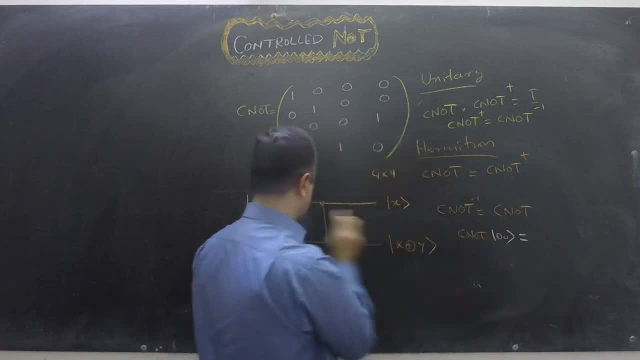 now, because the first qubit is 0 and the X qubit is 0, second qubit will remain the same, so our output will be cat 0- 0. if I have a CNOT gate and I applied that CNOT gate on qubits 1- 0, and because the first qubit is 1, so the second qubit will flip. 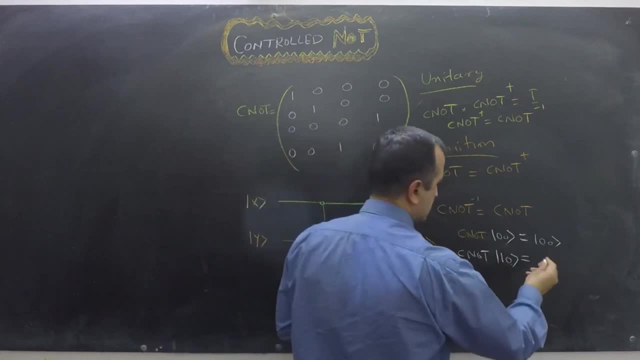 second qubit will become also 1, so my results going to be 1- 1. similarly, if I apply CNOT gate on cat 0- 1, then, because the first qubit is 0, my result will be 0- 1. and finally, if I apply CNOT gate on cat, 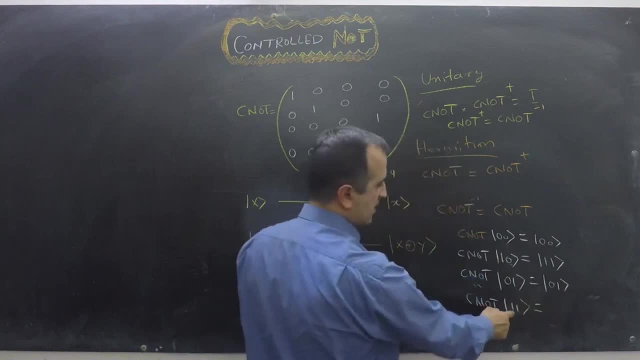 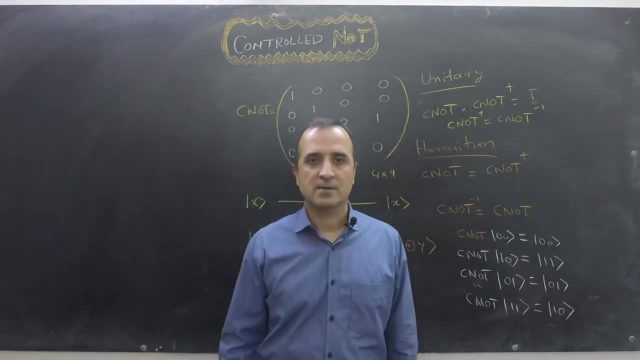 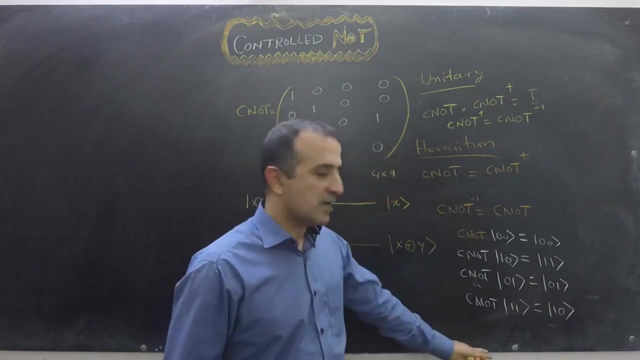 1, 1. then, because the first qubit is 1, so my second qubit will flip, so my result going to be 1: 0, because my aim is that everybody understand quantum computing. so instead of believing me that the results are correct, we should try out. 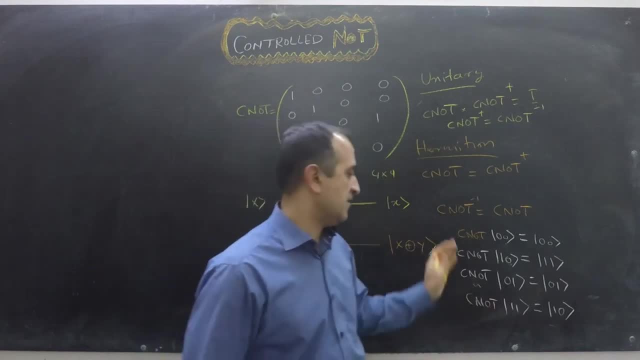 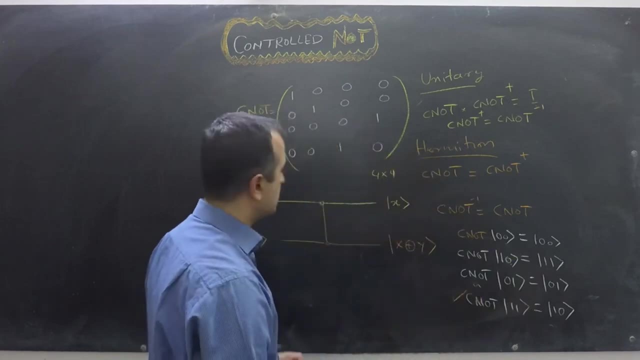 one of those results: using this matrix and verify if these results are correct. one of those result is: using this matrix and verify if these results are correct, correct, so maybe we should use this one. we should verify this result, so let's do that. oh so, I have made a one mistake here. 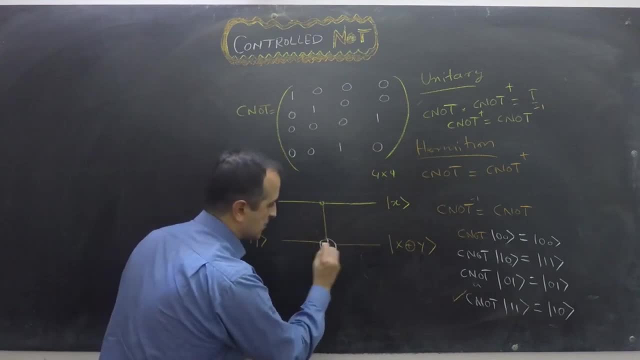 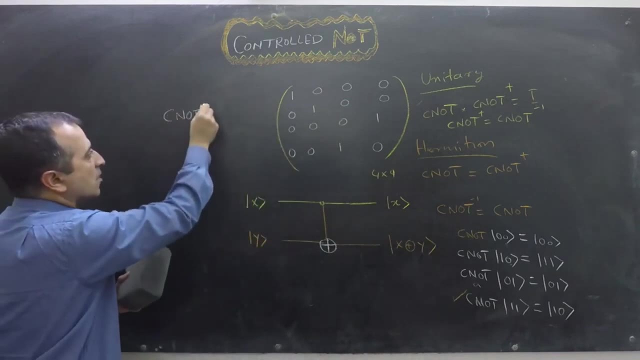 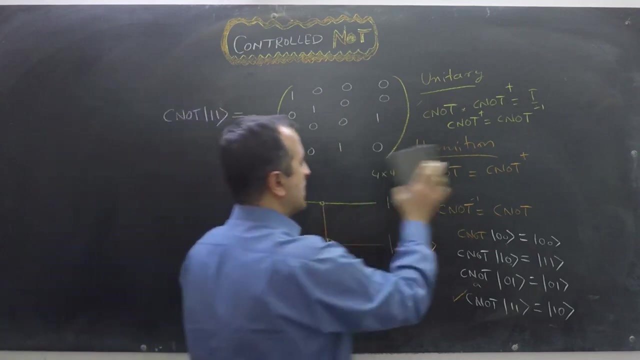 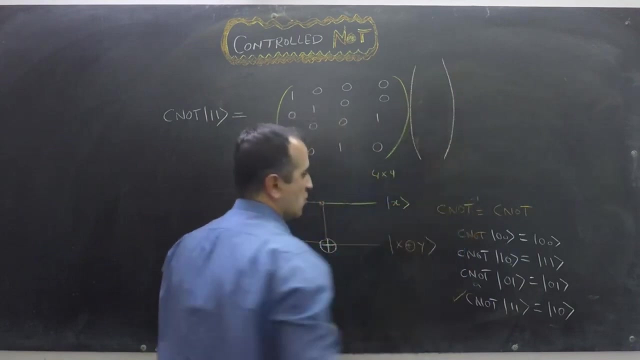 to have exclusive. so our goal is basically applying CNOT gate on cat 1: 1 and see what will be our result. this matrix represents CNOT gate and now we have to apply it and get 1- 1. so cat 1: 1 is going to be vector whose third. 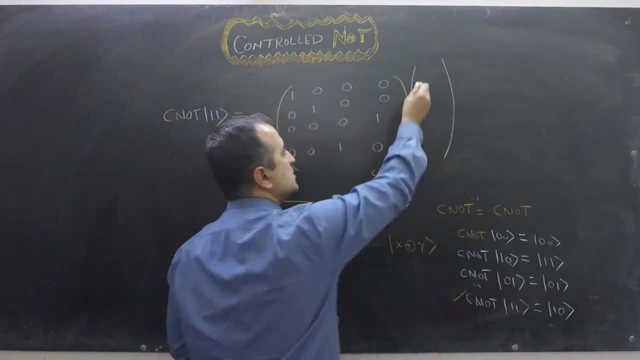 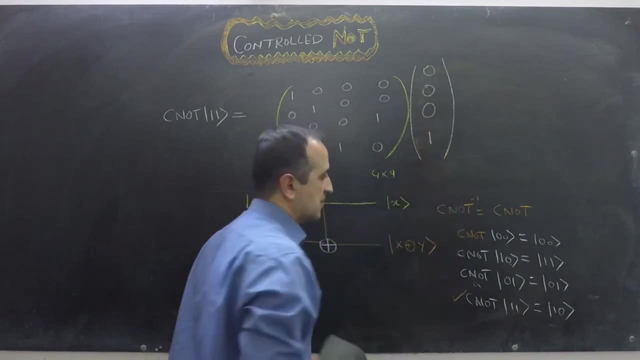 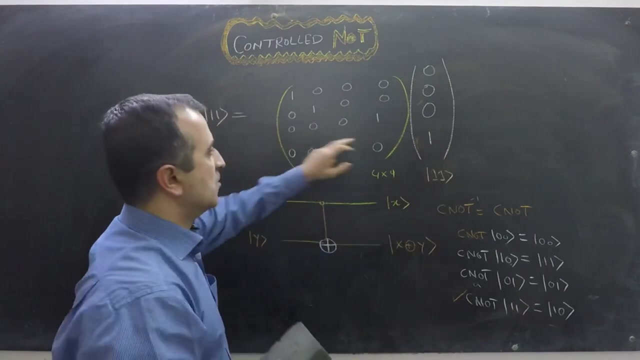 position will have 1 in it. so this is the 0th position of the vector. this is the first position of the vector. this is the second position of the vector. this is the third position. so this vector represent cat 1- 1. so we apply this matrix on this vector and see what will be our result, and 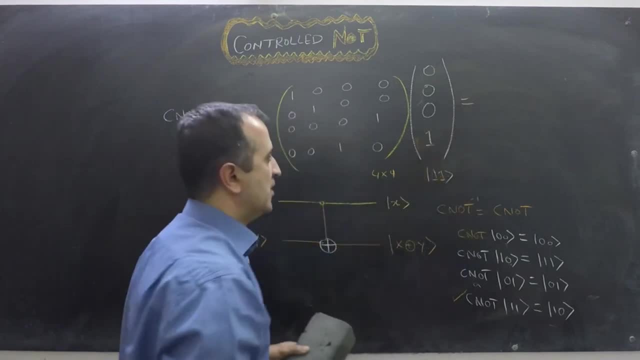 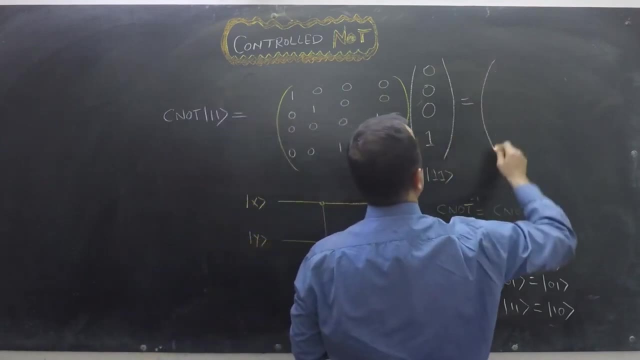 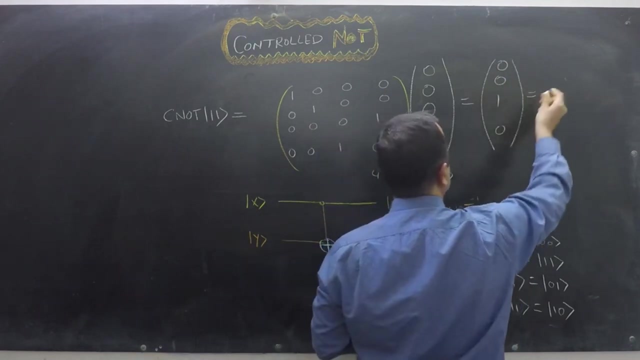 because the third position has 1 in it. so our result going to be this last third column, which is 0, 0, 1, 0. now the cost. a second position has 1, so we have to write 1, 0. that means 2, because second position has one in it. we. 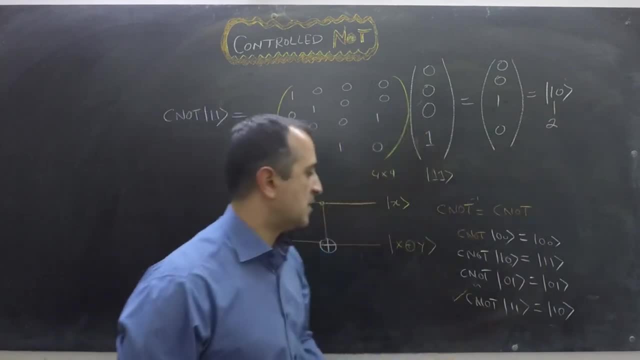 have verified that. indeed, when CNOT is being applied on get 1- 1, our answer is 2, because we want to apply it on our X2 cottage and that's true because ofл relatively. we have verified that. indeed, when CNOT is being applied on cat 1- 1, our answer is 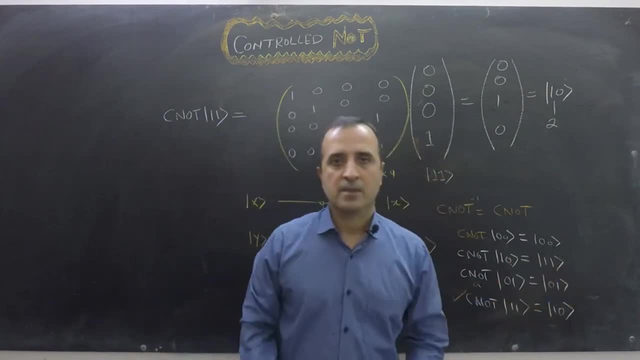 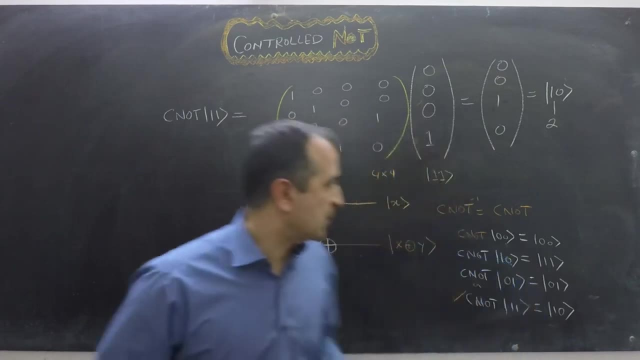 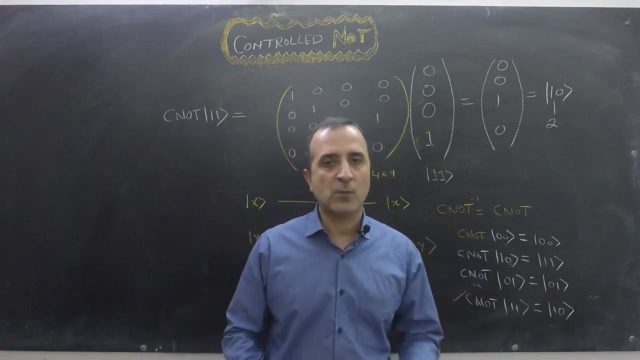 is ket01.. So far we have applied CNOT gate on pure states. That means this was a pure state of 00 and our result was a pure state of 01.. What if we apply CNOT gate not on a pure state but on superpositions, Like maybe we take ket0 and apply Hadamard gate? that 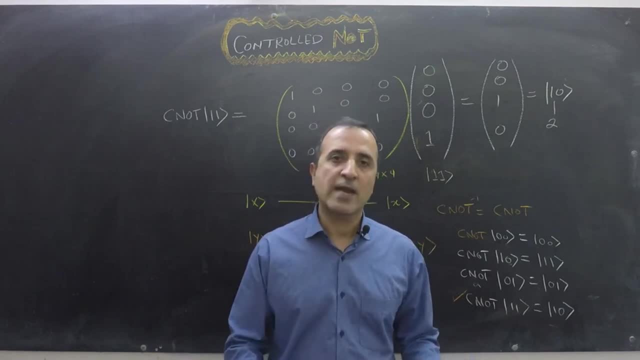 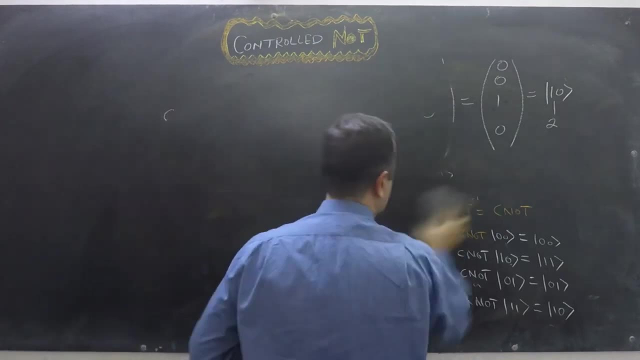 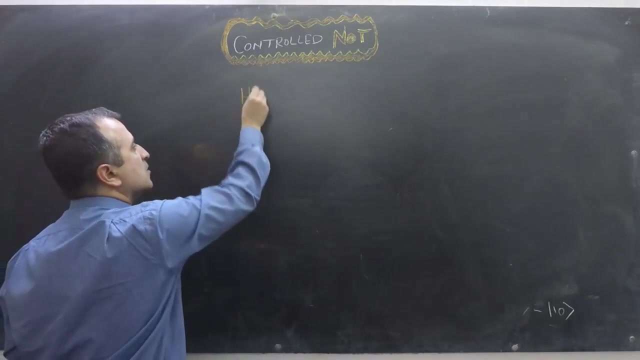 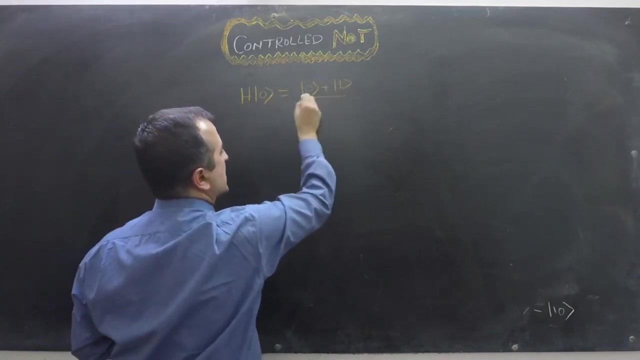 will create a equal superposition of 01 and we apply CNOT gate on that superposition. So let's try that out. So let me clear the board quickly. If we apply Hadamard gate on ket0, then our answer is ket0 plus ket1 divided by a scalar of 2, and this is referred to as 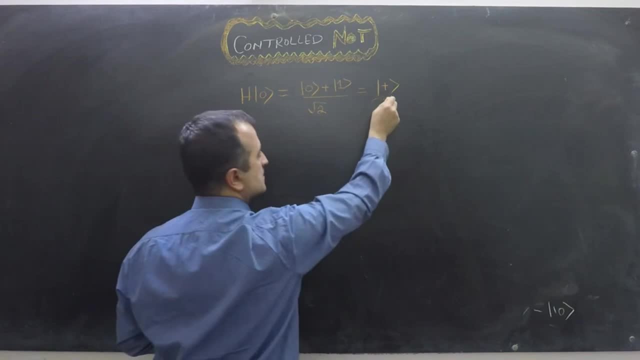 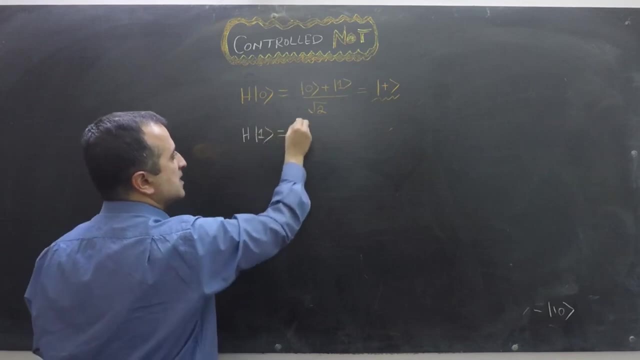 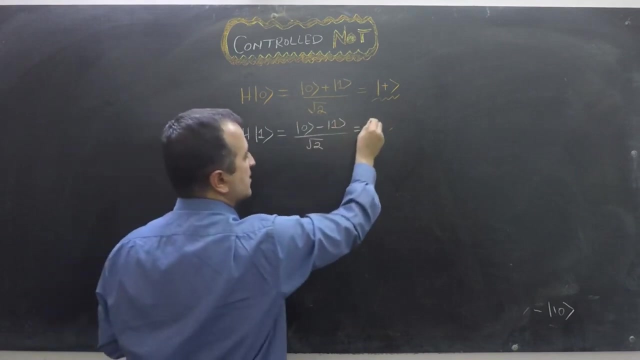 plus ket plus. Similarly, if we apply Hadamard gate on ket1, our answer is ket0 minus ket1 divided by a scalar of 2, and this is referred to as minus, ket minus. So let's say we have a CNOT gate. 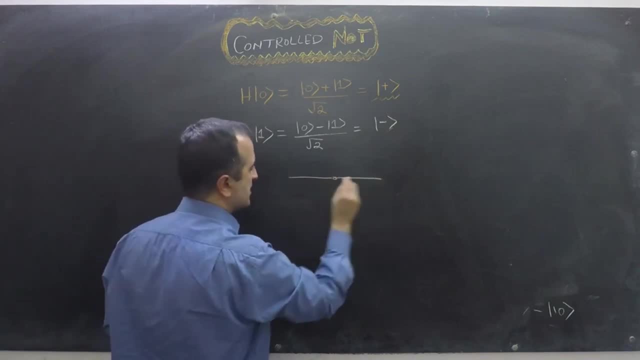 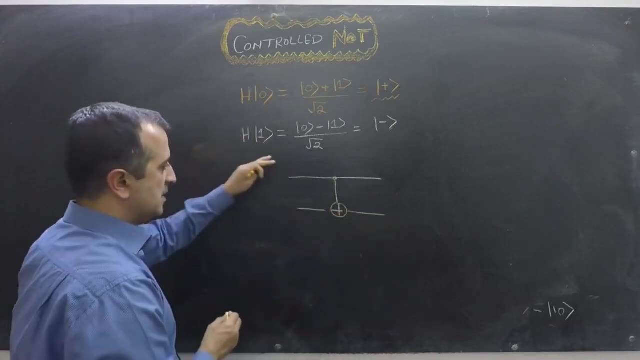 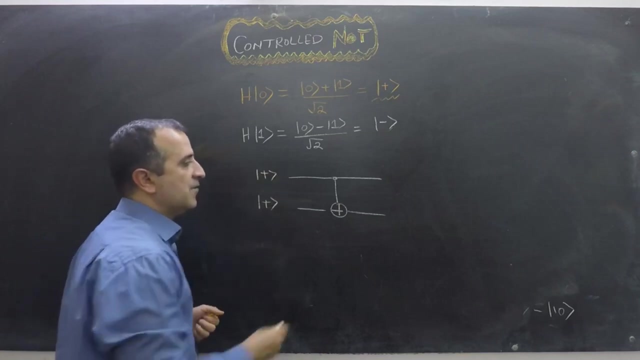 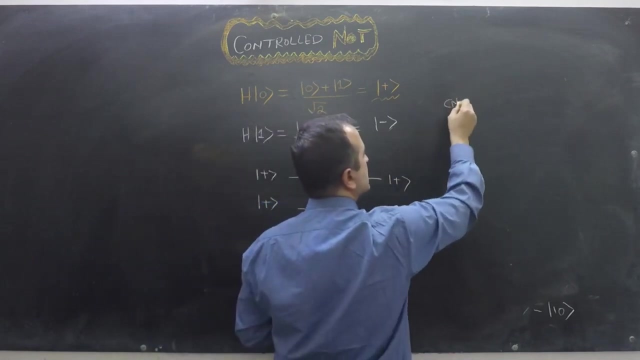 here. This is our CNOT gate. Instead of giving that gate some pure state, we give it ket plus and ket plus. Then our result is ket plus and ket plus. So let's say, if we apply CNOT gate on ket plus, ket plus, our result is: 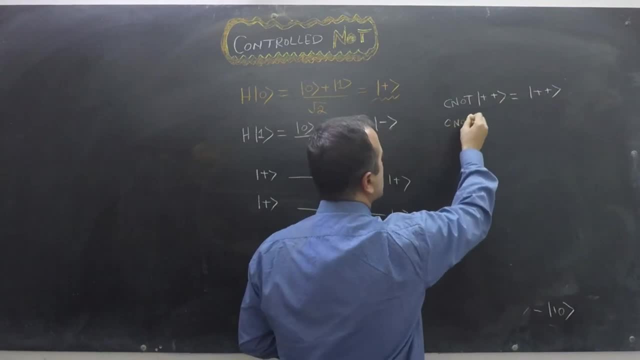 ket plus, ket plus. If you apply CNOT gate on ket minus ket1, together with our pad on our sub invector, that means this is target of啦. the user get minus plus, our result is minus plus. so the rule is this in this case. if the second qubit is: 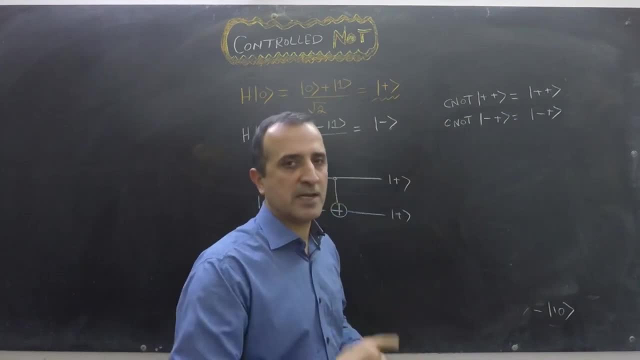 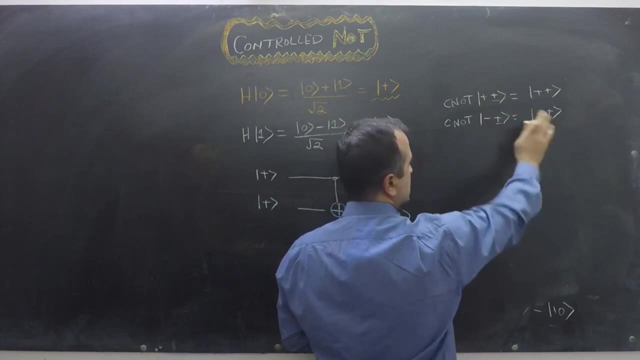 minus, then the first qubit flips from plus to minus and minus to plus. so in the in this case, because the second qubit was plus here and plus here, so our result was remains the same. but what if our second qubit is minus? that means we have minus minus. then the first qubit will flip. so we 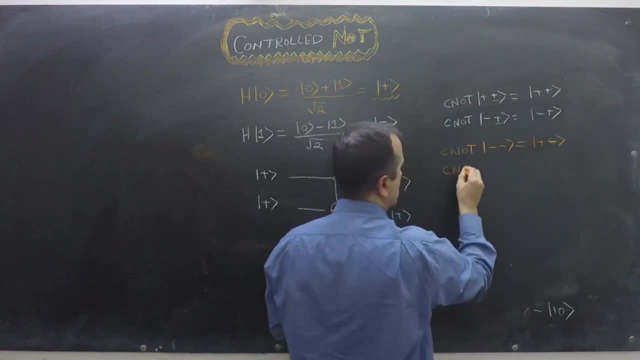 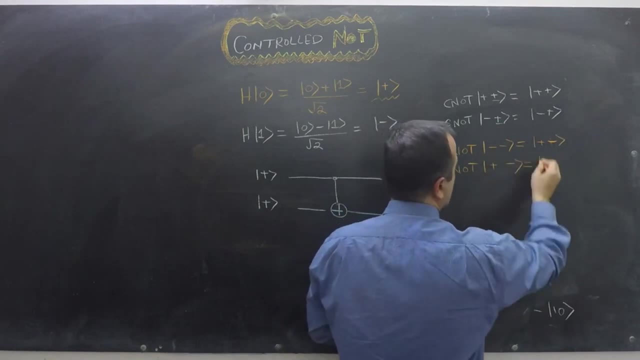 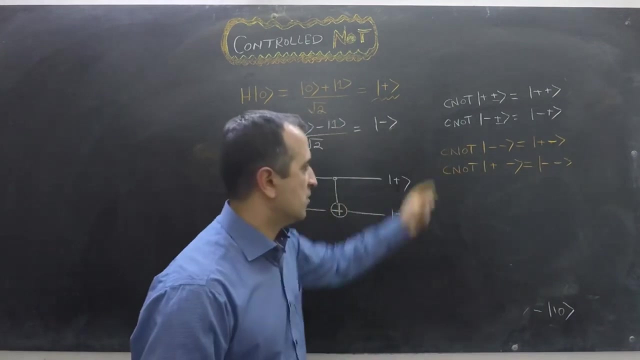 will have plus minus. similarly, if we have apply C node gate on, second qubit is minus, first qubit is plus, then our first qubit will flip to minus, so we will have minus- minus. maybe we should also verify one of those result for the sake of our practice. so let's say which one we should verify. 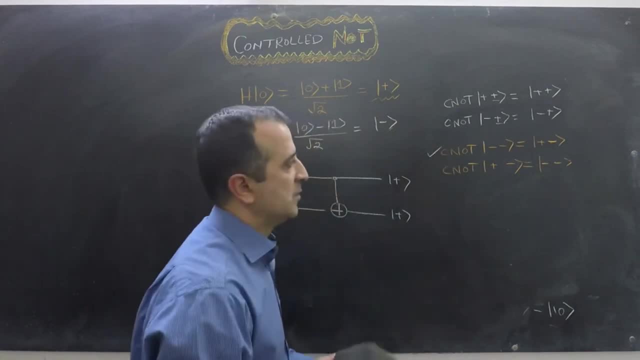 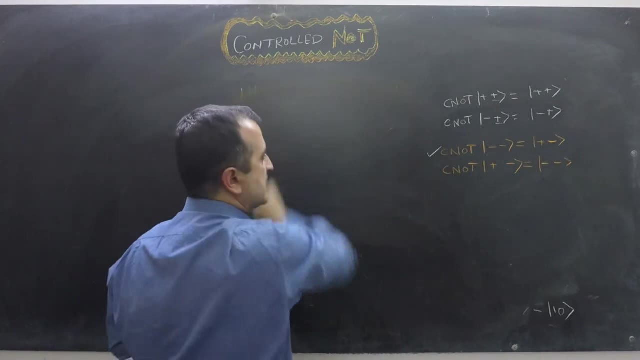 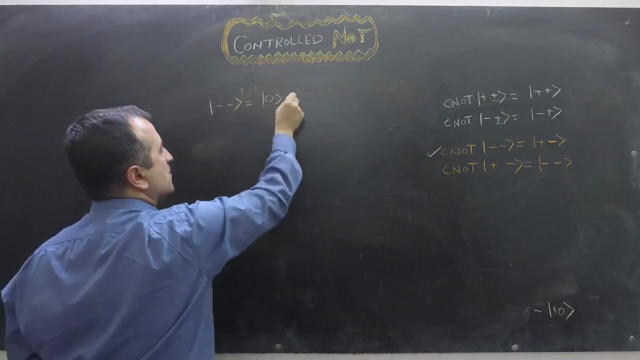 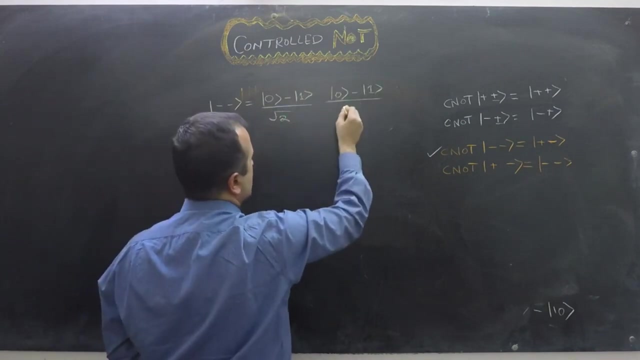 maybe we should verify this. this one looks difficult because they are flipping and both qubits are minus minus, so let's try this one. so first figure out that what is cat minus minus? cat minus minus is equals to cat zero minus cat one divided by a square root of two times cat zero, cat one divided by a square root of two. and. 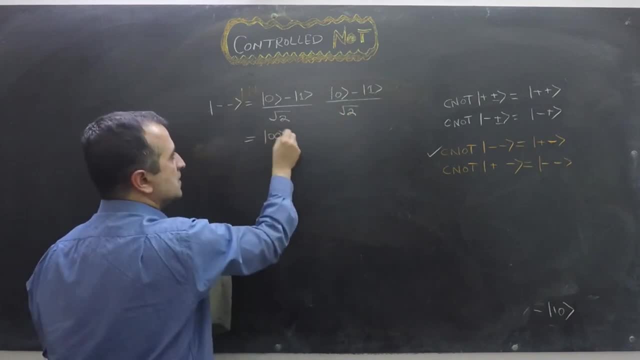 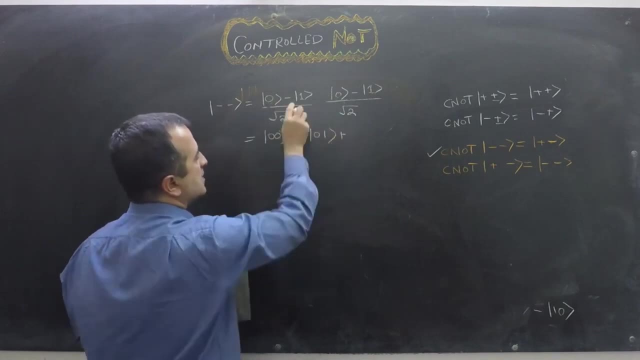 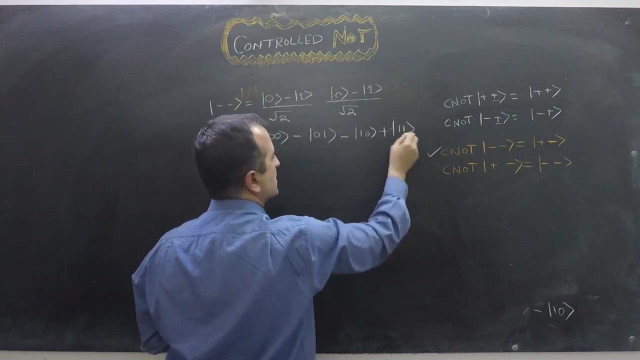 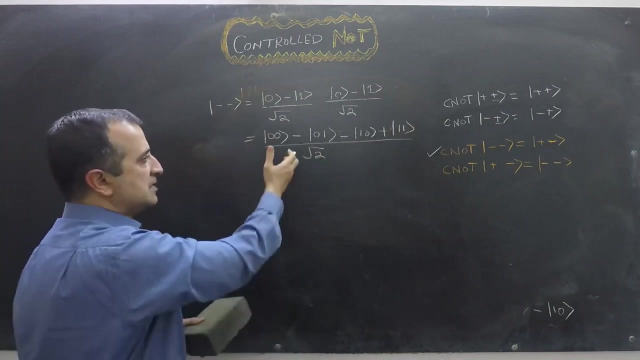 when we simplify it, then we will have zero- zero because this and minus zero one. we will have then one zero and finally we will have plus one, one divided by a square root of two. now, because we want to verify it using matrix, so we have to convert this in the form of vector, so in the 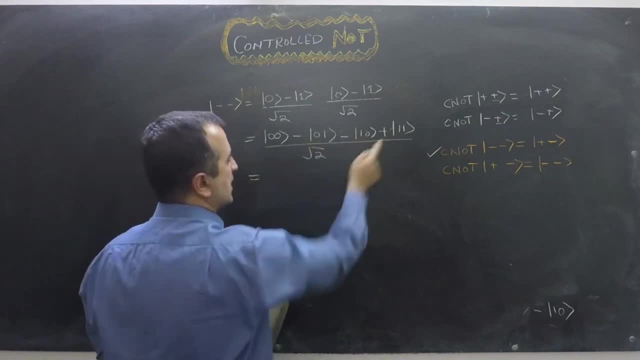 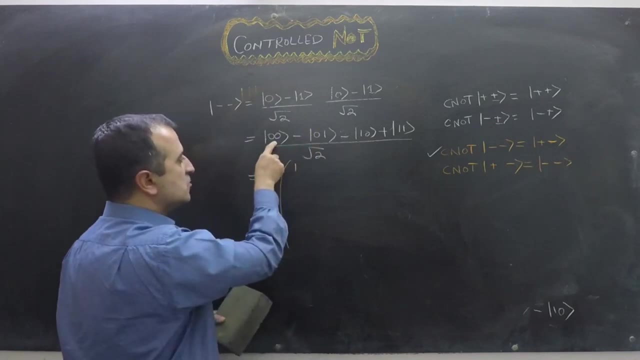 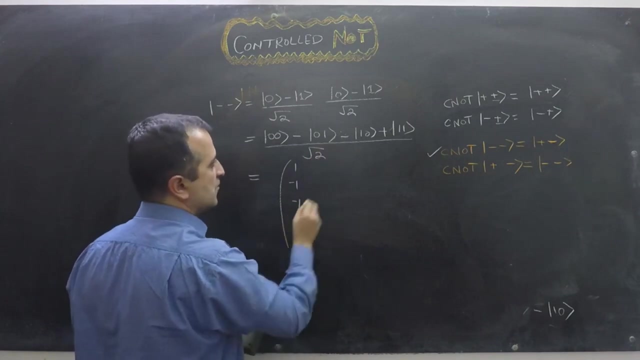 form of vector. we will have one on all of those places and the signs will be whatever the sign we have. so we will have plus one for for the zeroth location, we have minus one for the first location, we will have minus one for the second location and we have plus one for the last. 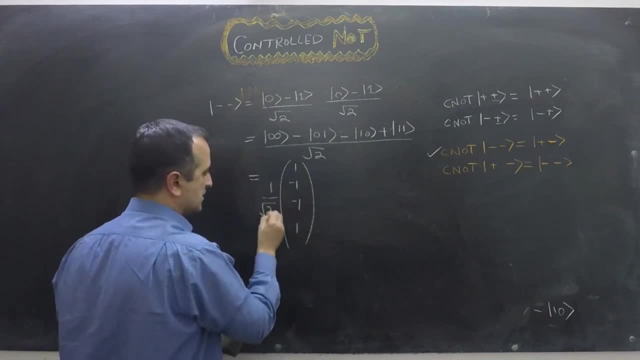 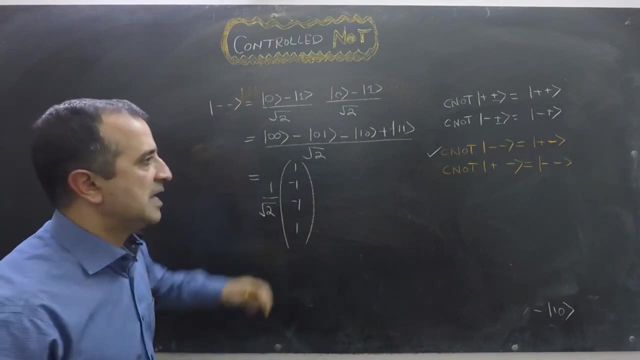 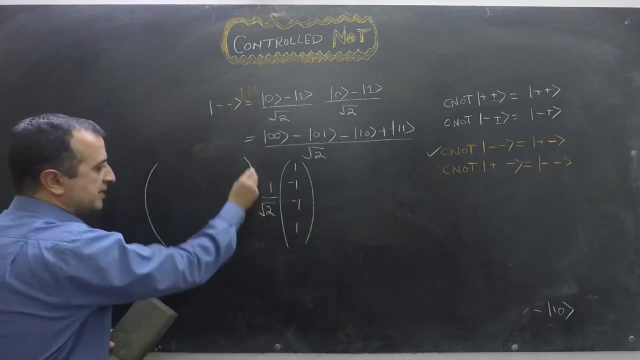 location and we will have one over scale of two outside. this is our vector and we have to see if we apply our c naught matrix on this vector, if our result is equal to this or not. so let's apply c naught matrix on this vector. our c naught matrix is one zero, zero, zero, zero, zero, one, zero zero. 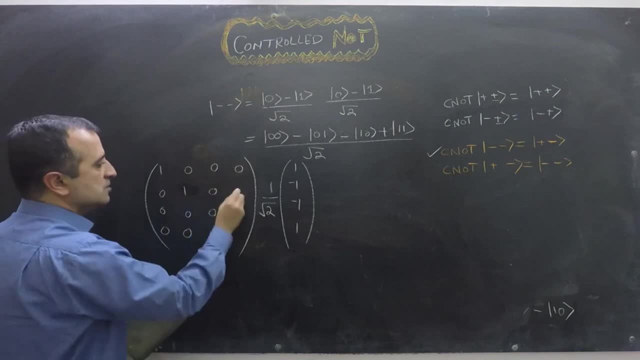 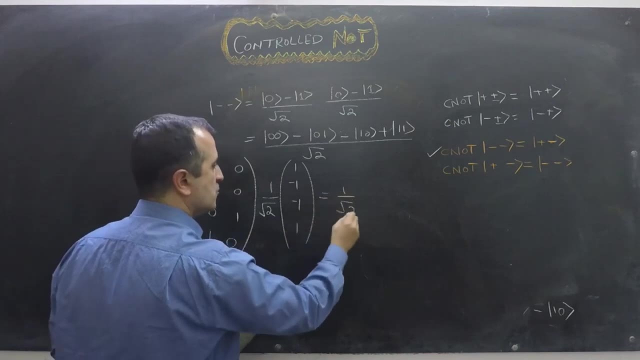 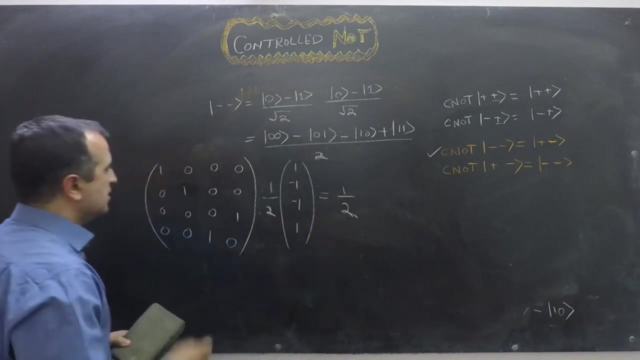 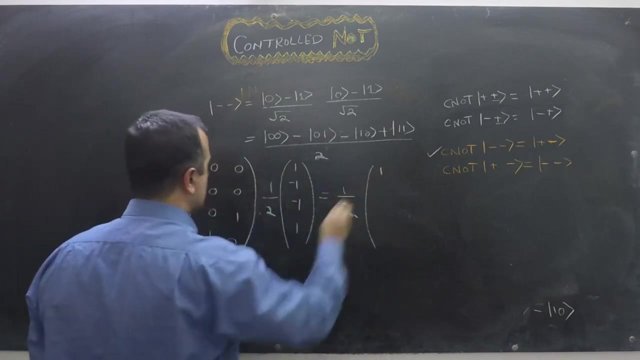 zero, zero, zero, one, zero, zero, one, zero. we apply our c naught matrix on this vector, we will have one over square root of two outside. I think if we made a mistake it should be one over two- and then we apply this thing to this and we will get our one. we apply this thing to this, we will get minus one. 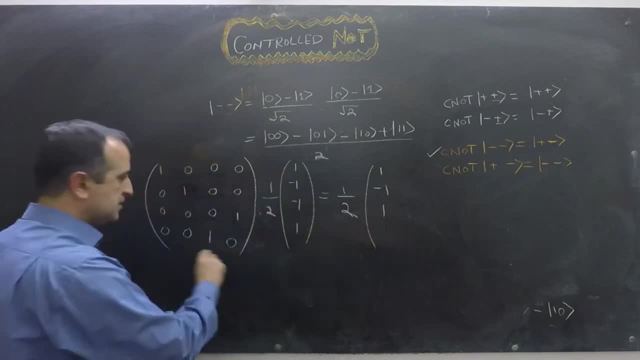 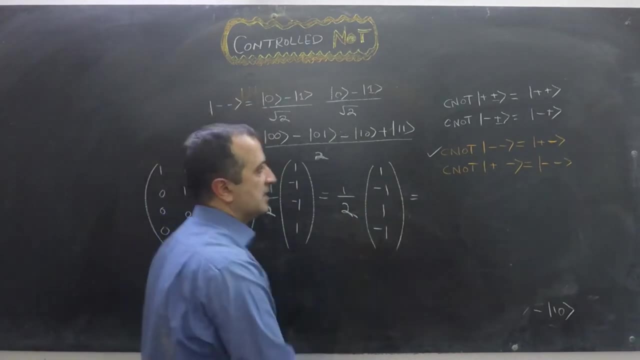 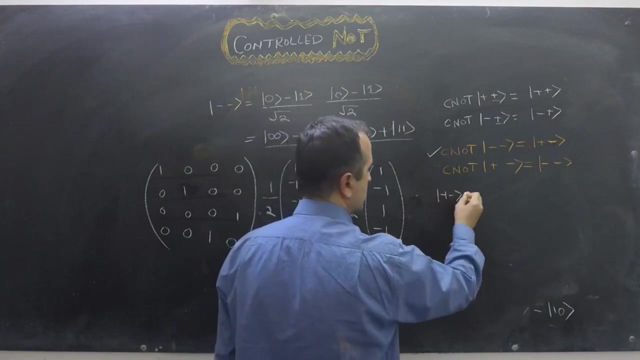 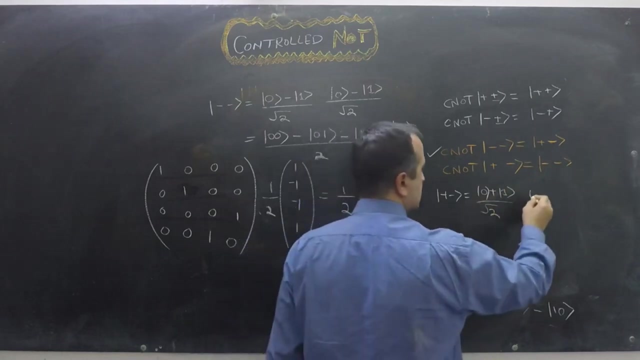 to this, we will get one. we apply this to this: we get minus one. if our result is correct, if this vector is equals to plus minus- and let's check, check this out- so we know that plus minus is going to be cat zero plus cat one, divided by square root of two times cat zero minus cat one. 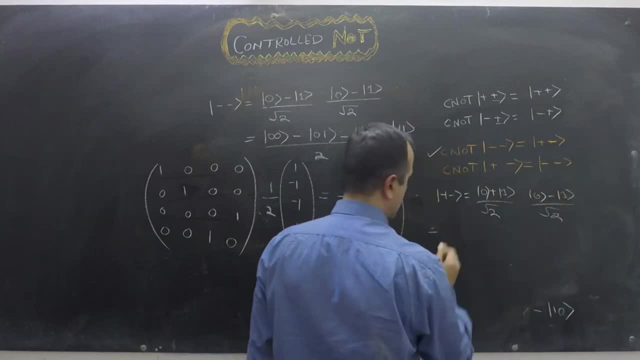 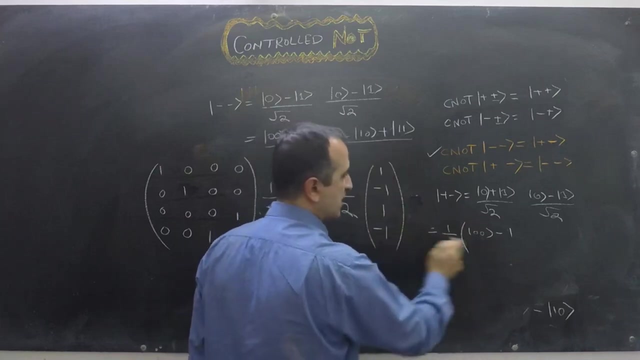 divided by square root of two and we will get one over two outside and inside. we're going to get cat zero zero minus cat cat. so far we are right, because first location will have plus one and we have one over two outside and second location going to have cat zero one. so this is sorry, this is zero location. this is first location. 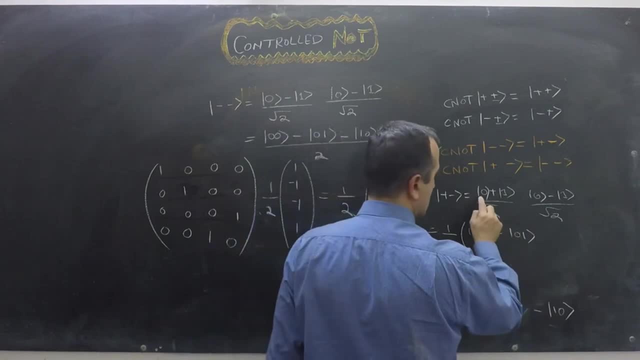 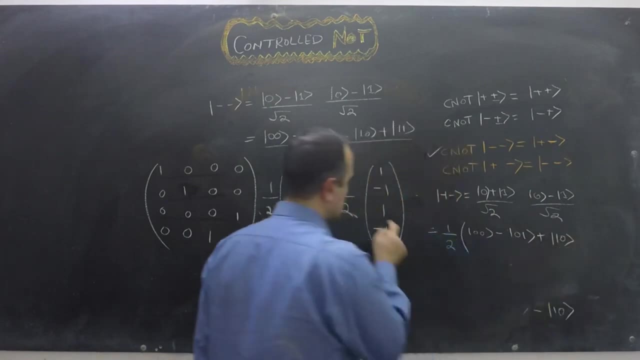 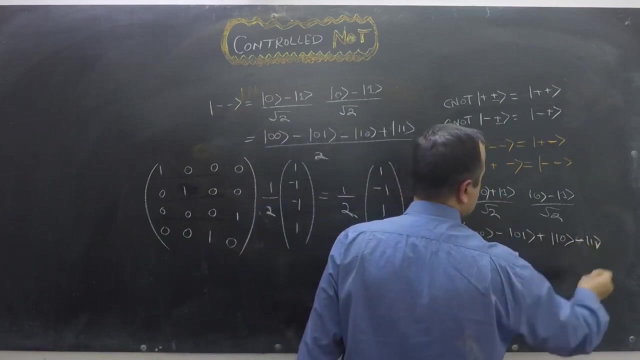 that it is indeed minus one, that this is correct. also, now we multiply this with this, we get plus cat one, zero. and third should be plus one. this is correct. and the last going to be minus one one, and this is also correct because the last location will have minus. so we have verified that. when we apply c,